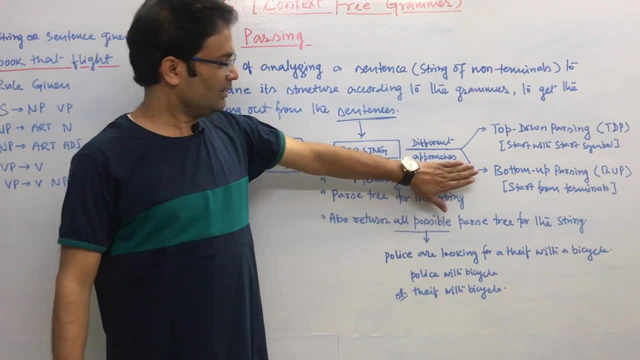 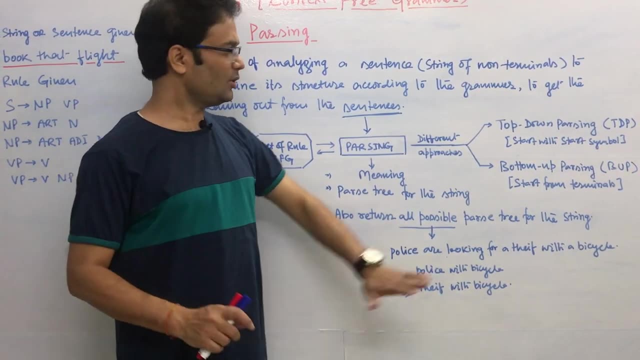 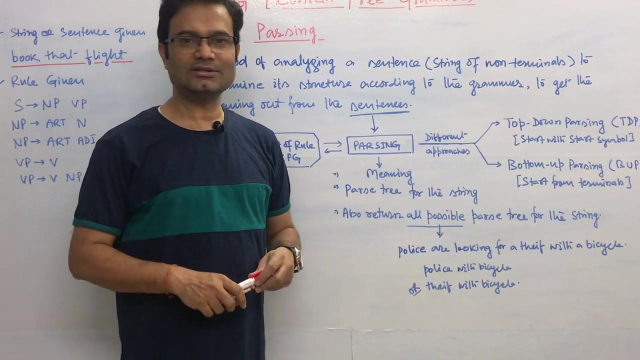 symbol, what is the terminal, what is the non-terminal? And when you use the bottom-up parsing that is called the BUP will be start from the terminal. But the purpose of the both approach would be the same. we have to find out the parse tree from the given sentence. 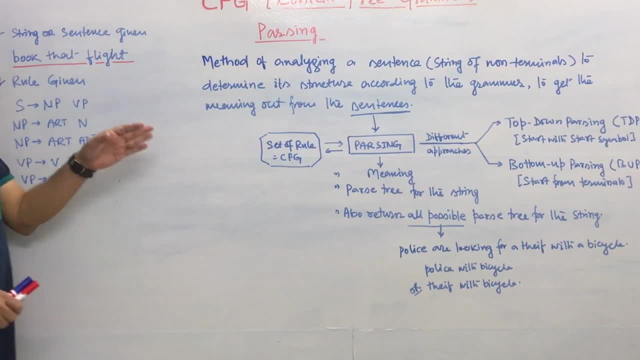 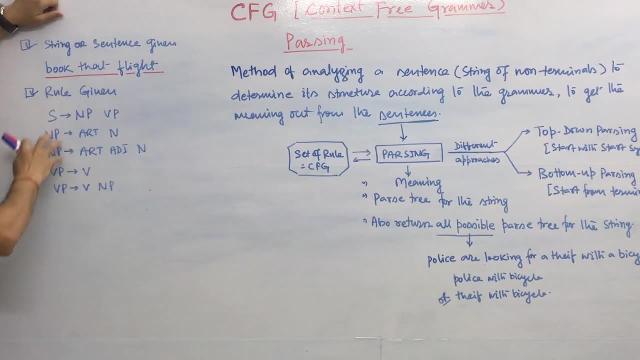 with the help of the CFG. So suppose, So suppose, Suppose, if one sentence has been given, that sentence is called the book that write and the CFG rule is also given means in this case this is given, and this is given we have. 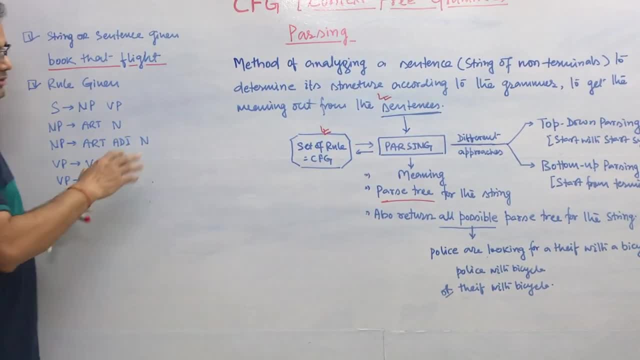 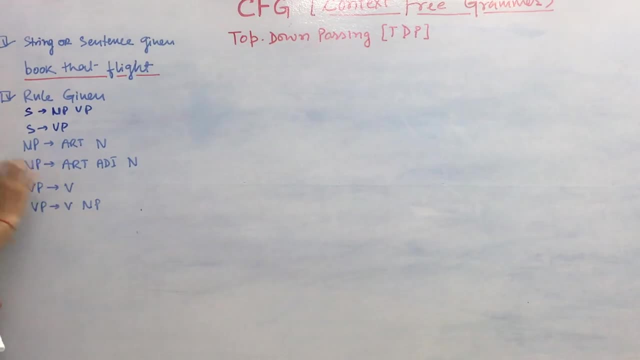 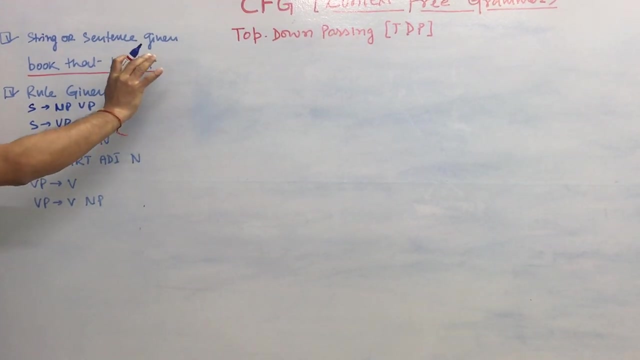 to draw the parse tree. So let us draw the parse tree. first we take the top down. parsing sentence has been given book that write and these are the rules. So what I will do, I will take the rules and check whether that rule is applicable. of the 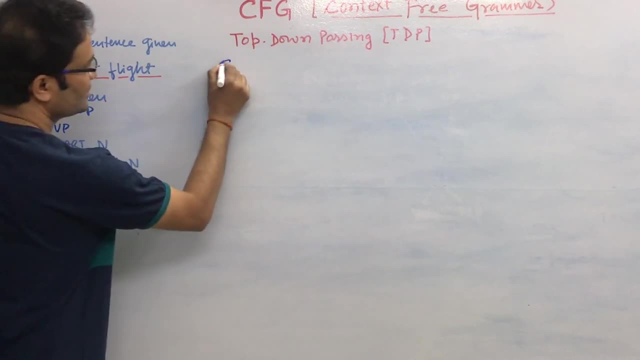 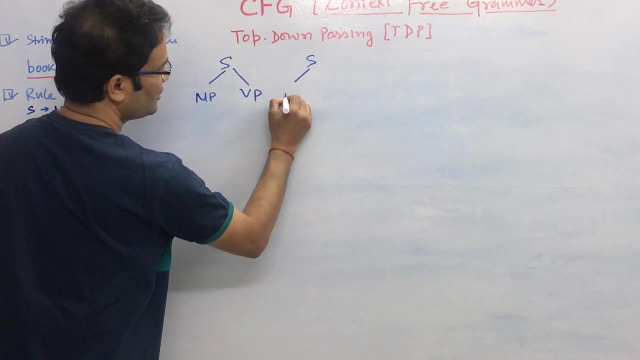 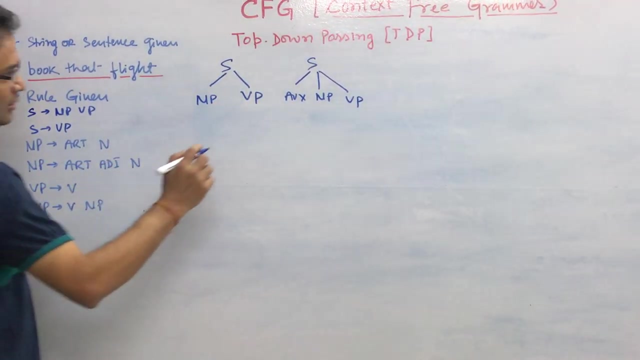 given sentence or not. So take the first rule as noun phase and the verb phase. another set of rules is that auxiliary noun phase and verb phase. that is not there, but this is a common one. Third, take the as and the verb phase. 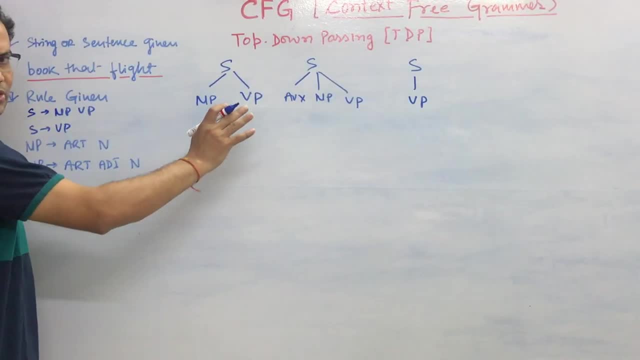 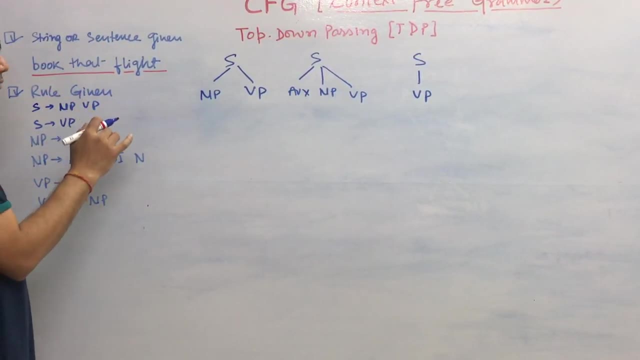 As and the verb phase As and the verb phase. Now check whether which is going to suitable according to the given sentence. So here we know we are taking the top down approach. so we know what is this book? book is the verb here, this is not the noun. 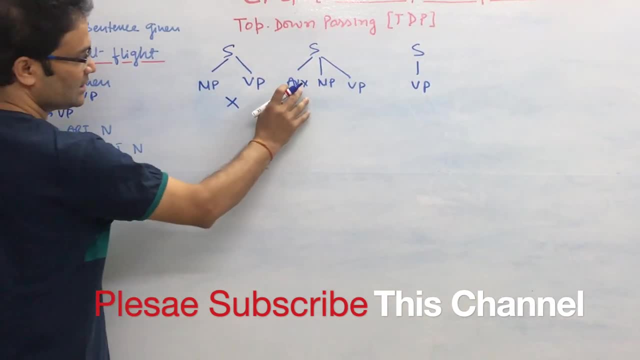 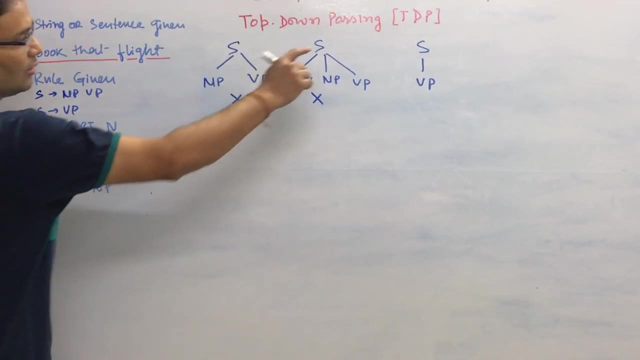 So this is the ruled out. it will not work. Second case: before noun: you could have any auxiliary. So even I do not have the nouns, we are not going to take it Now. the starting symbol and the verb phase: It is matching here, wait. 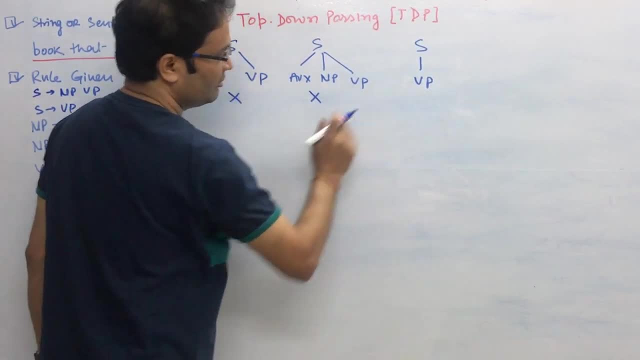 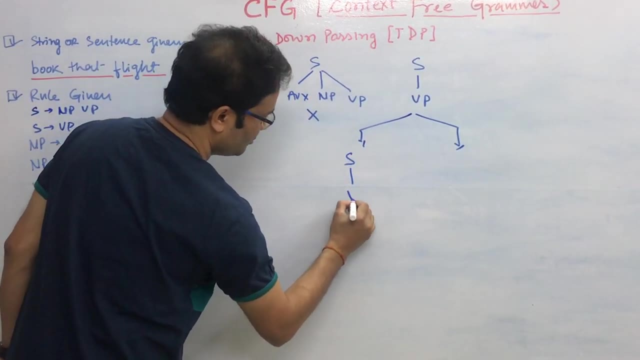 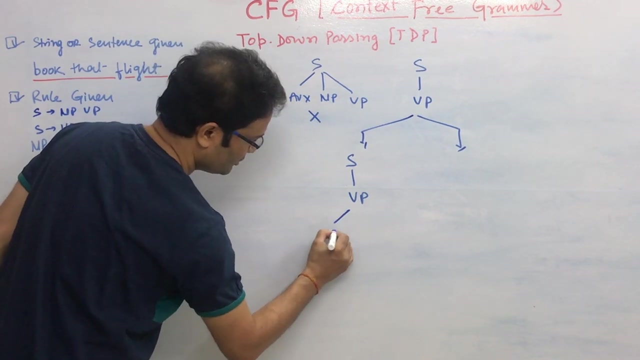 So now take the further, decompose the verb phase. So there are the two approach here. One approach, verb phase, and if you see the verb phase, we have the two part verb and the noun phase, verb and the noun phase and we have verb phase on a singular verb. 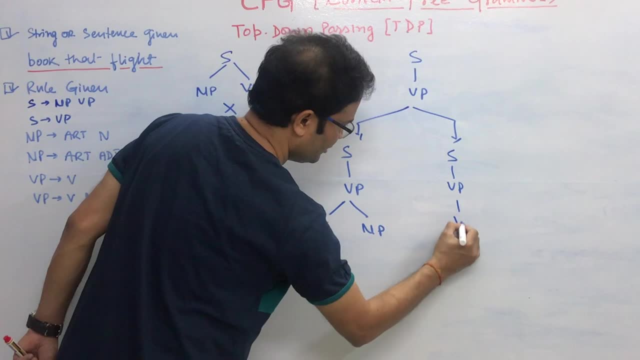 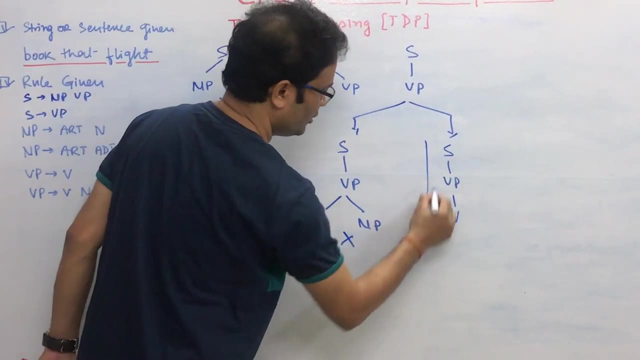 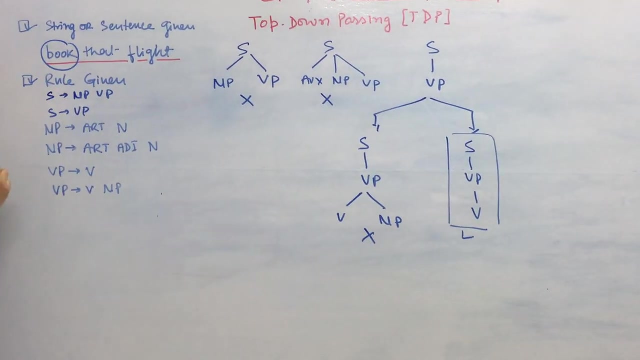 So as verb phase and the verb. So we do not have this condition with you, right? So this is ruled out, So we have this one. So now we finalize this part, right? So with this part, this is ok, ok. 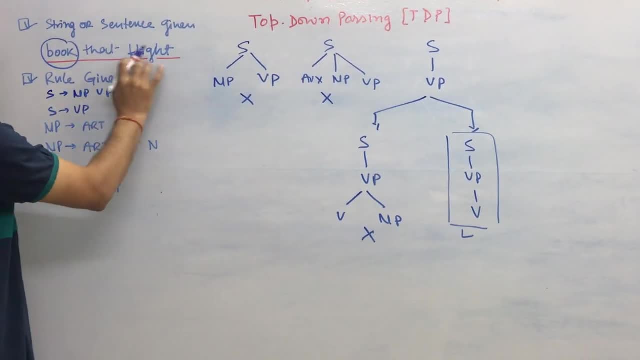 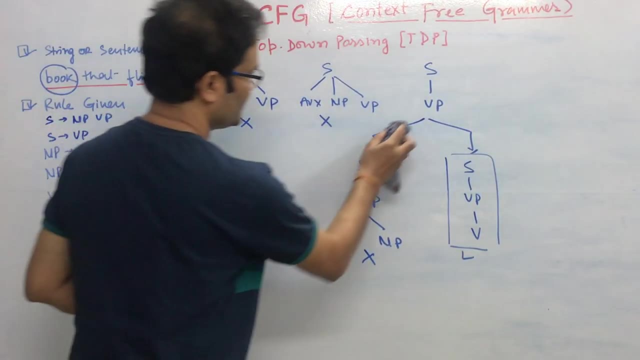 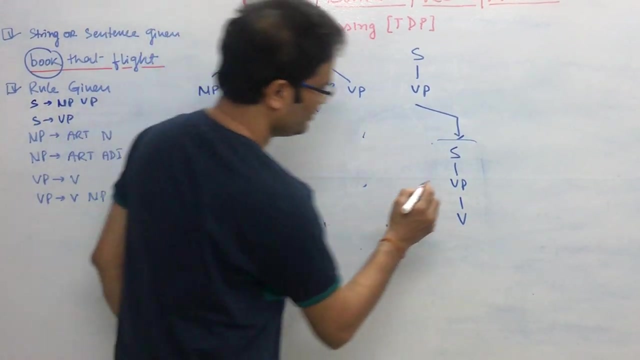 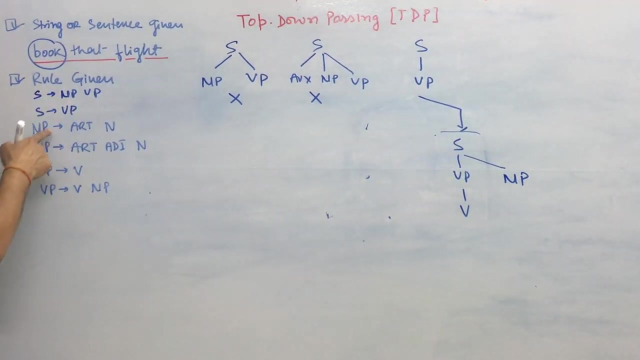 Now we have to use that other part. So other part is that the this is the noun verb, noun phase, right? So so this part is conformed. Now, second part is we take the noun phase, and noun phase is include the alt key and 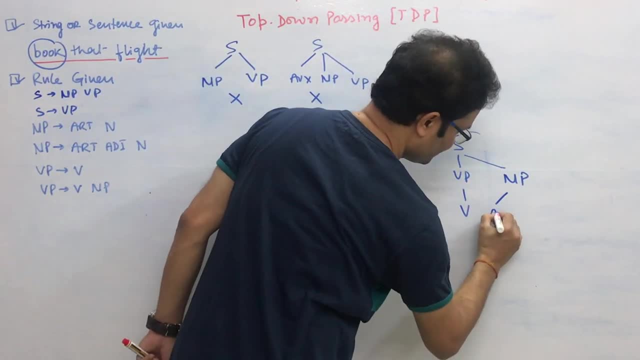 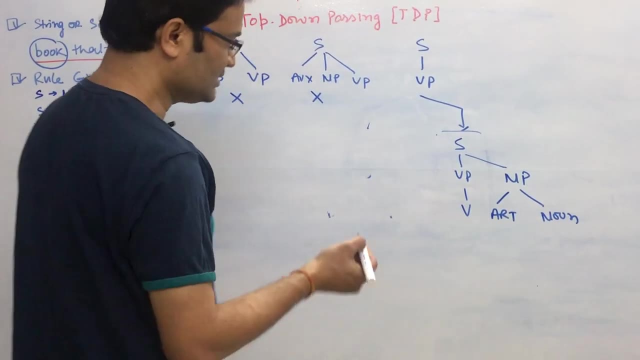 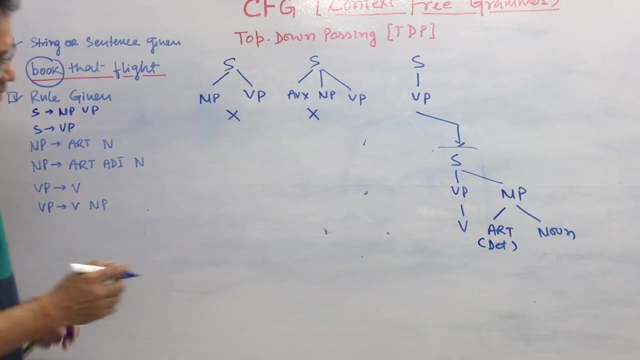 the noun right. So we will take the alt key and the noun right And you can say the alt key and you can also say the determinant. both are same right. So now try to set: Is everything ok? Is everything is setting or not? 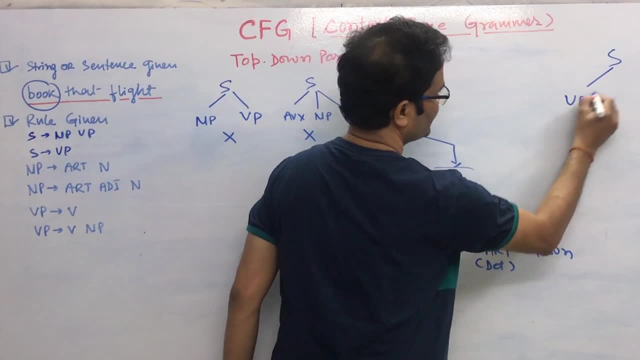 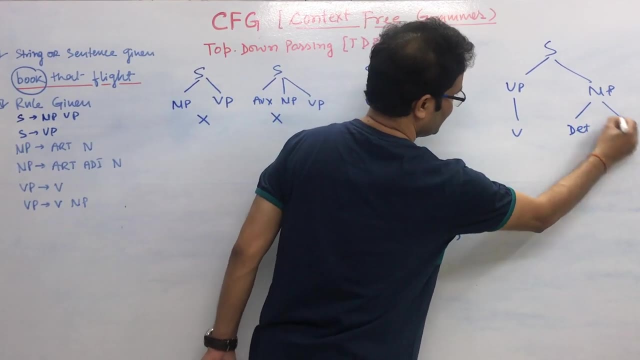 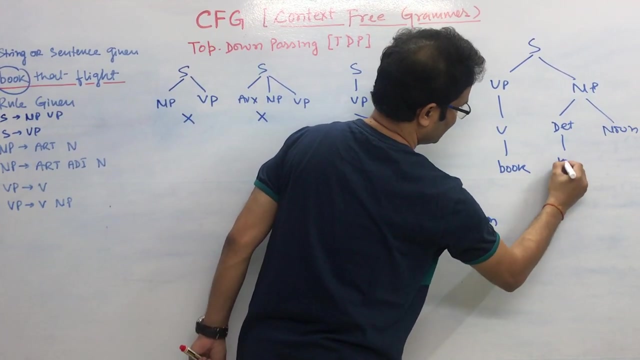 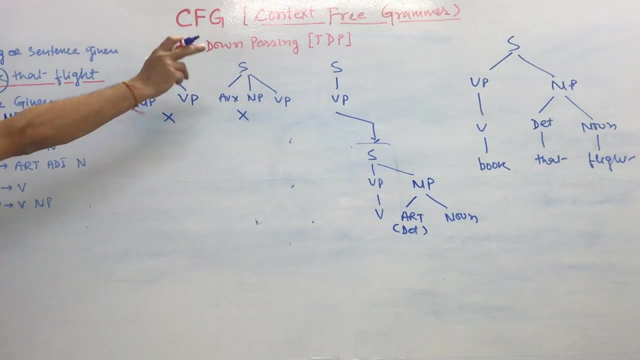 So, as we have taken, then the verb phase, then the noun phase, with this verb verb is coming, here is the determinant is coming, here is the noun is coming for the verb book determinant that, and this is the right. So that is the top down parsing for this given sentence. 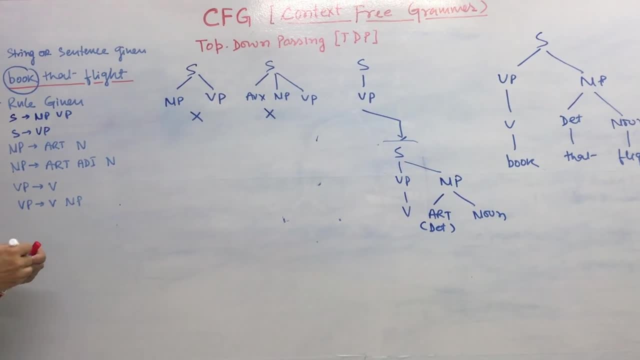 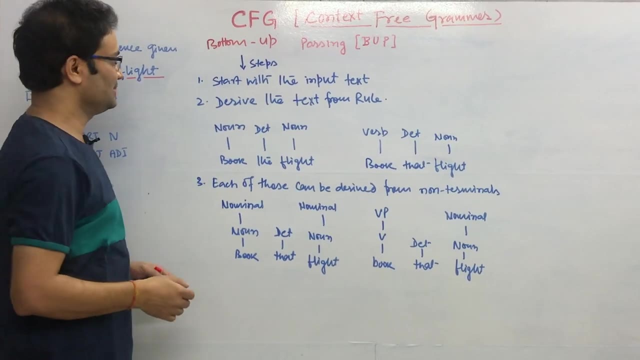 Now let us see the next part. This is the way we do that. So if you do the practice, we can just understand. this is not the big thing. Now let me at the bottom of approach. So we have to take some few steps. 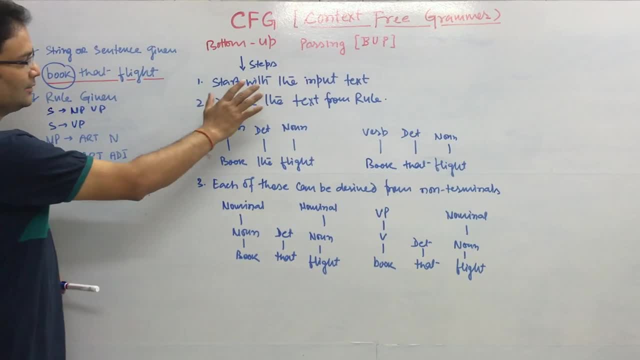 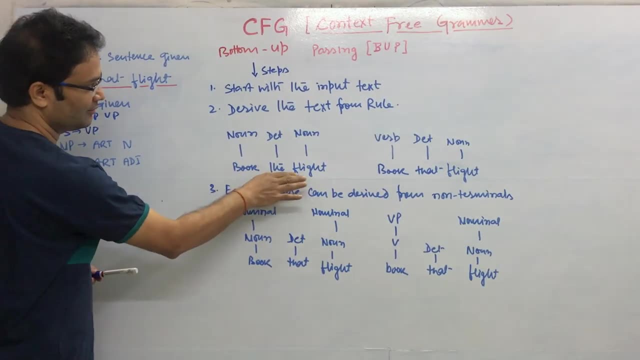 So we start with the given input sentence: book that flight. Now we have to derive the text from the rules. So this is my text: book the flight. So, as per the rules, we can just derive. So: book is the noun, the is the determinant and flight is the noun right. 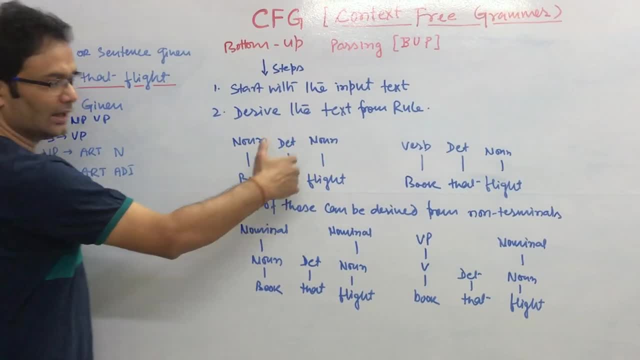 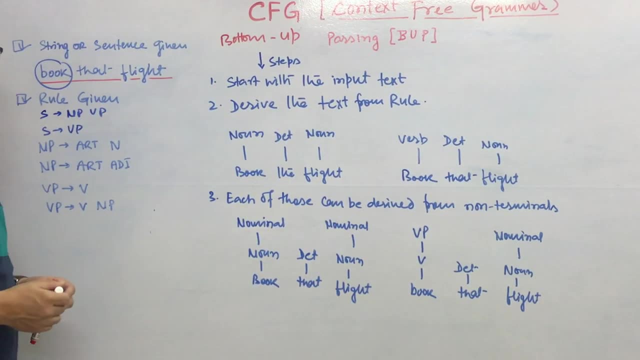 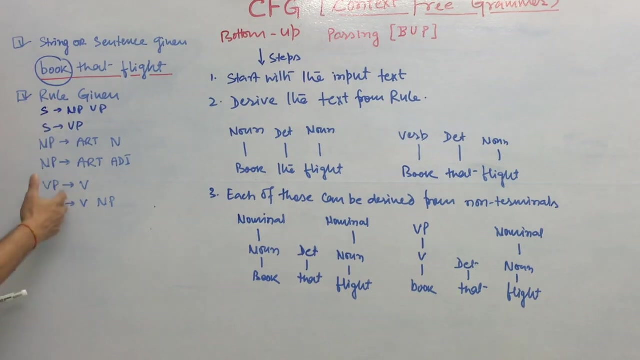 And we have to write the text. So we have to write the text, So we have to write the text. And other possibilities would be there. book could be the verb and the determinant and the noun. right Now we have to derive, we have to use the non-terminal also, as you have seen, that rules 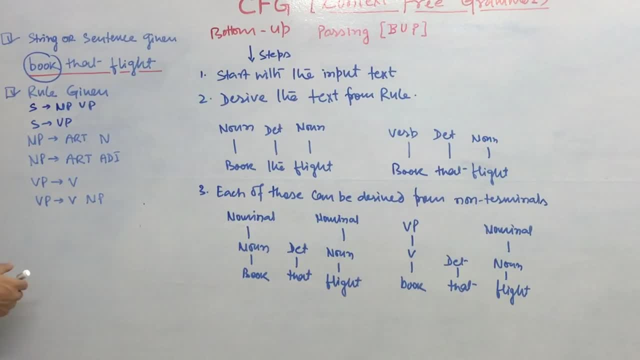 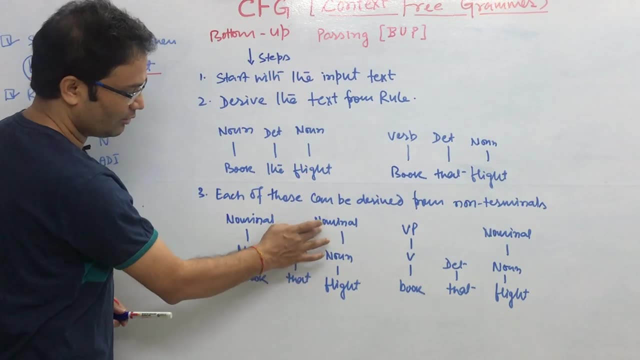 So if you derive something bottom that should come from the non-terminal, So let us noun for the noun, we can take the non-terminals: nominal For the noun, also non-terminal For the verb, for noun, also nominal. So let us use the non-terminals.